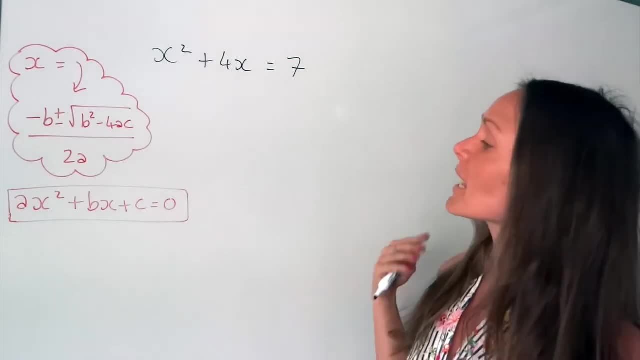 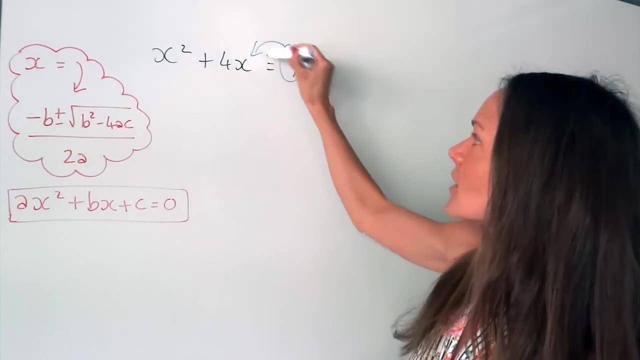 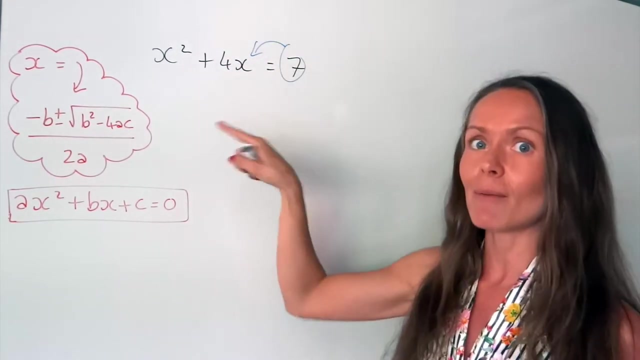 So if we look at this example here, it doesn't say equals 0, like it should, So we need to start by moving that 7 over to the other side. Okay, so remember, when something moves across the equal sign, it changes sign. So this positive 7 will now become negative. So I'm just going. 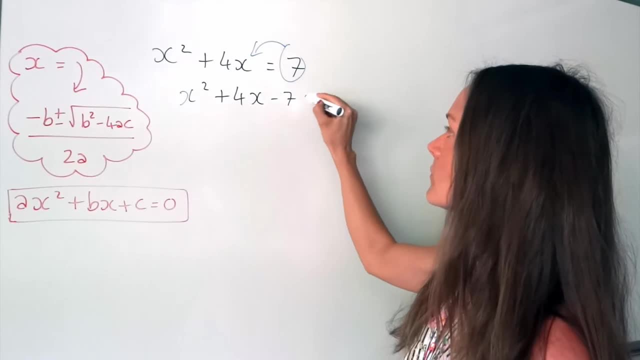 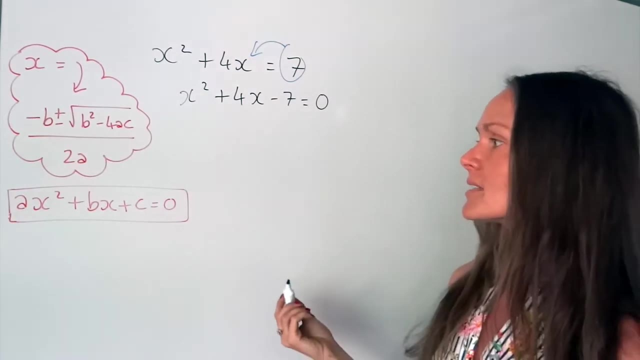 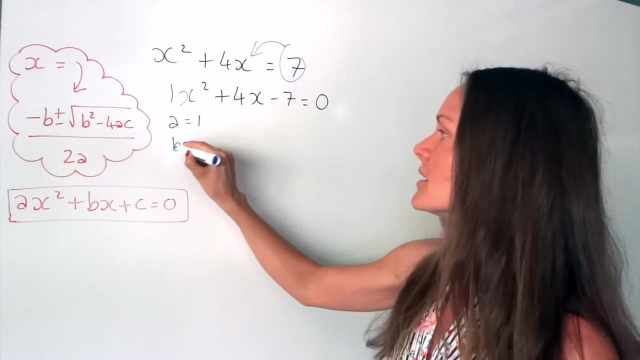 to write out that new equation down there. Okay, so now let's identify our values: a, b and c. So remember a. A is the number in front of the x squared well, here there's like an invisible 1, so a is 1.. b is the number in front of the x, so positive, 4.. Don't forget to look at the. 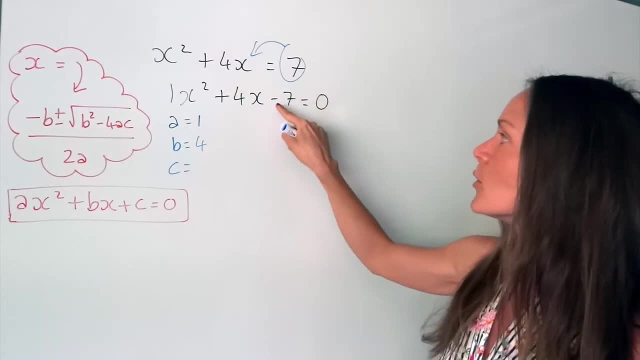 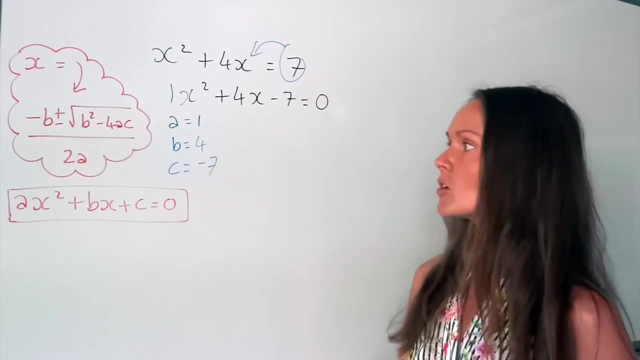 sign And c is the number by itself, which is this 1, so negative 7.. So now that I've identified a, b and c, it's just substitution. You're just substituting these values into this formula. So in the calculator you would put: 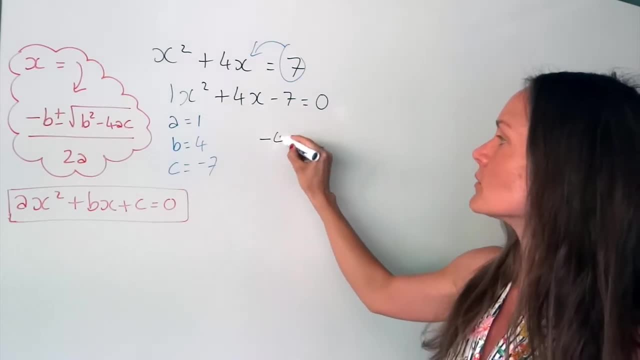 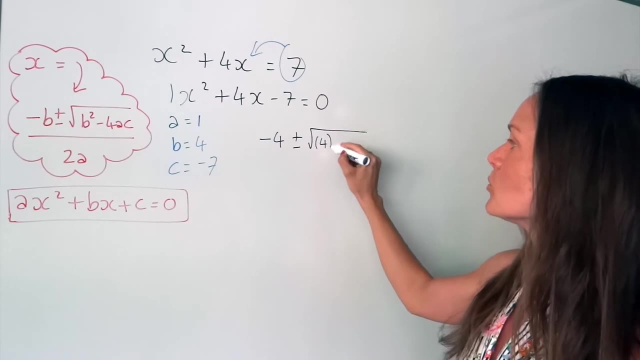 Nice. minus b, so minus 4, plus or minus the square root of b squared, so that would be 4 squared, and I'm going to put that in brackets and I'll tell you why later. and then minus 4 times a. 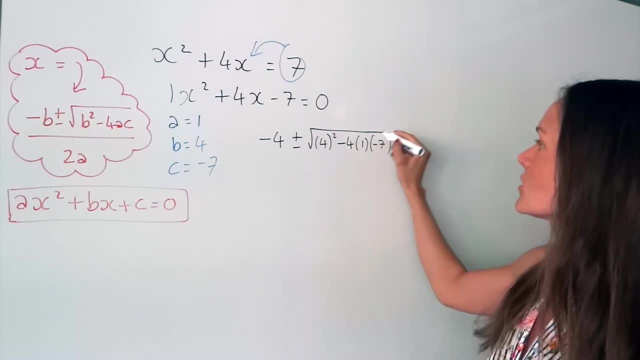 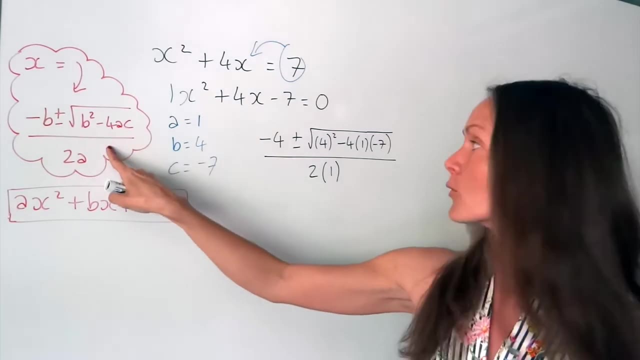 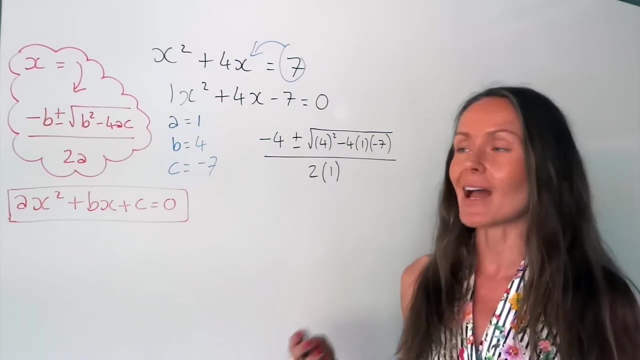 times c. So I'm literally just swapping in all those values a, b and c. okay, So I'm putting these into this formula. Now I would always put brackets around these numbers, because some people don't put brackets. and if this was a negative value, if you did negative, 4 squared like this: 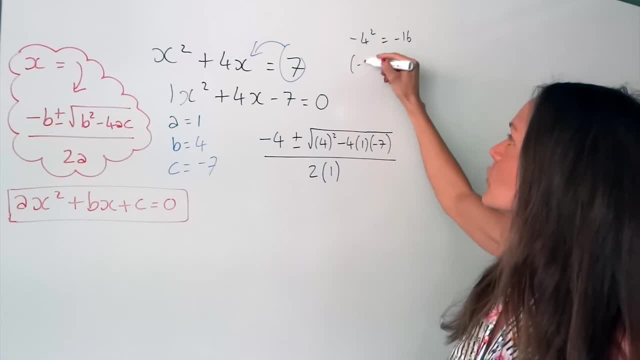 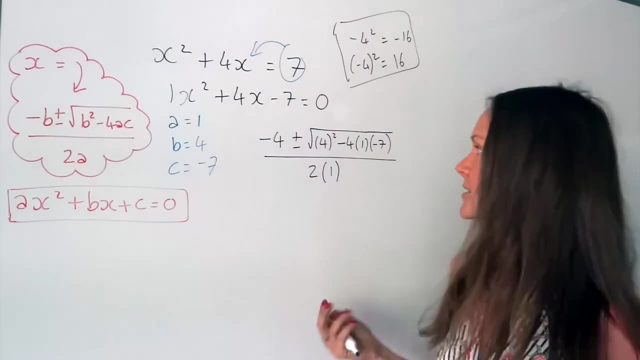 without brackets it gives you minus 16, but if you do it with brackets it gives you positive 16.. So it's always a good idea to put your numbers into brackets, like I've done here. It's just a good habit to get into. So put that in your calculator. so press your fraction. 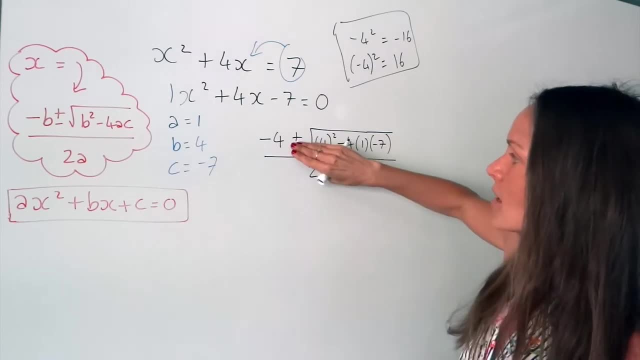 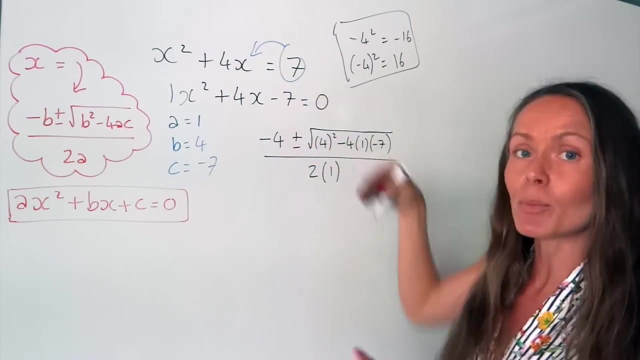 button then type it all in. Once you do with plus, okay, you press equals, you can keep it on your screen, then you can go back, delete the plus and change it to a minus, because remember, when you're solving a quadratic equation, there are two solutions. All right, so let's see what. 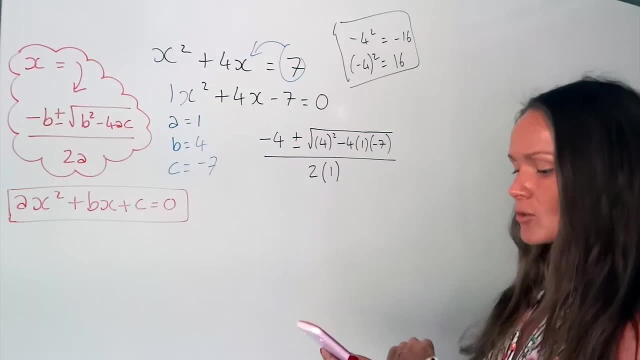 we get, and if you've got a calculator you can do it at the same time, just to make sure you've got the same answer. So I'm doing it with plus to start with and my first answer when it's plus, if I 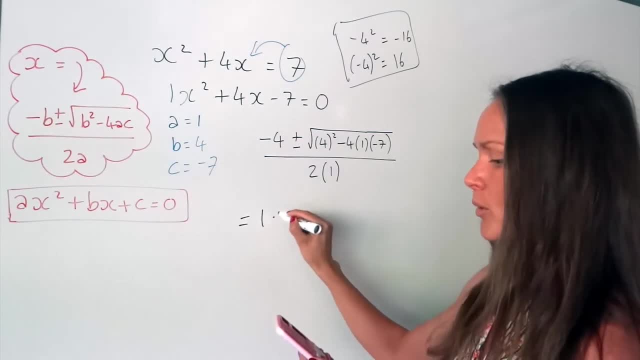 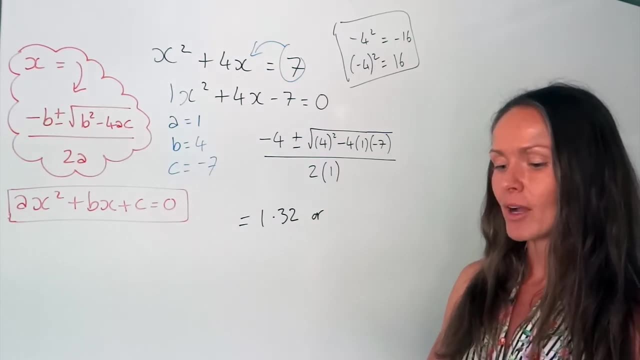 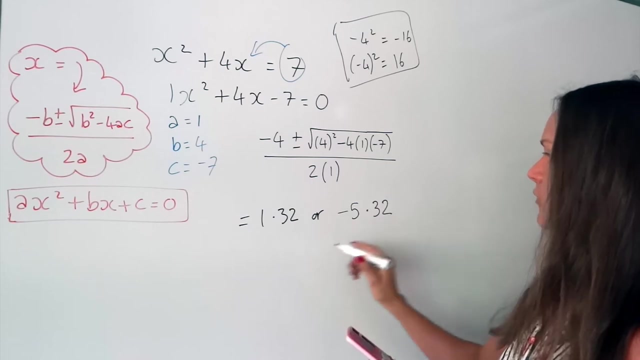 round to three significant figures is 1.32.. Now, just like I said, leave the answer on your screen and just backtrack, delete that plus symbol and change it to a minus, and then my other value, if I round to three significant figures, is minus 5.32.. Hopefully you got the. 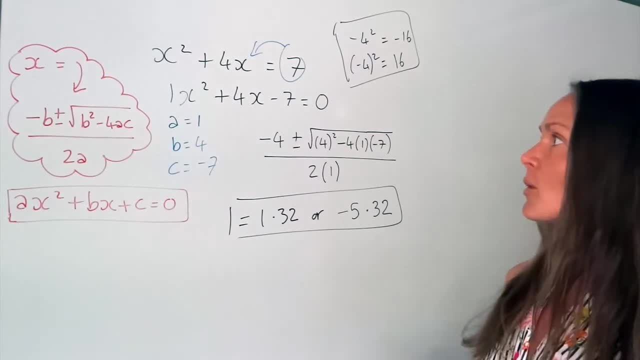 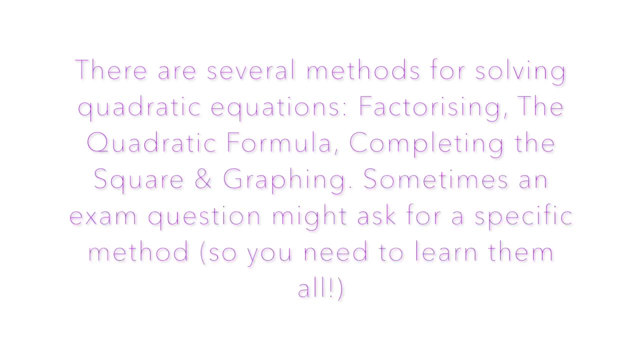 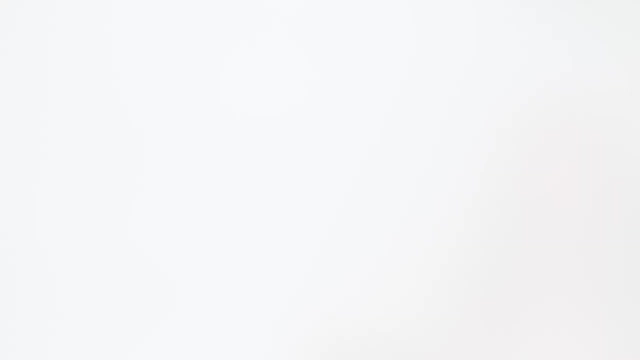 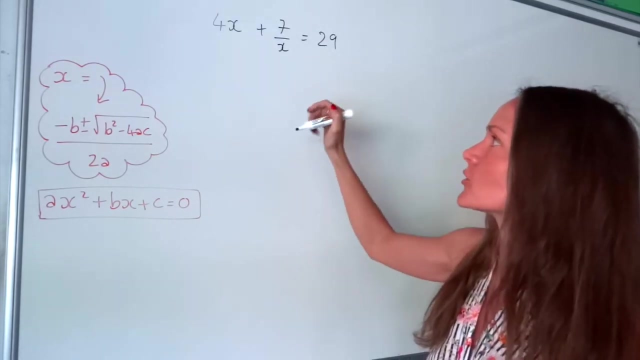 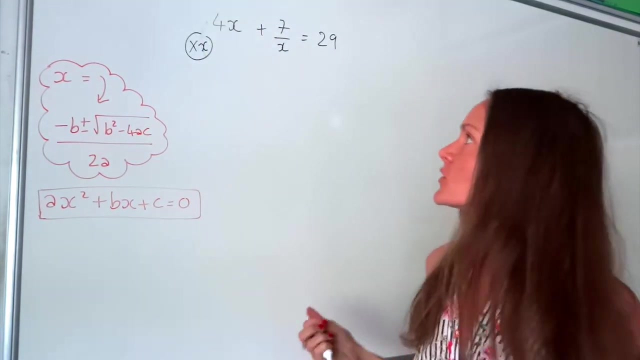 same if you did that on your calculator just now as well. I'm going to do a hard one just to finish. Okay, so my first step in this one is to get rid of this fraction, because I don't want x in the denominator of a fraction. So I'm going to multiply everything in this equation by x. So if 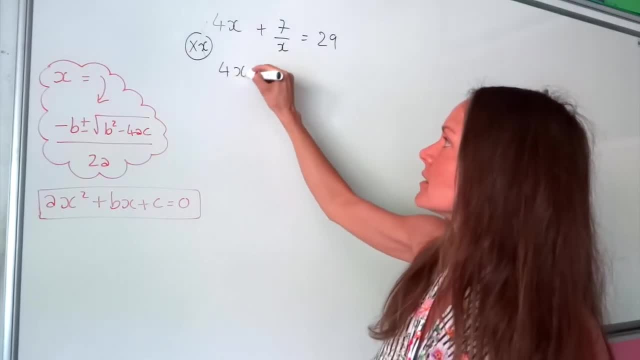 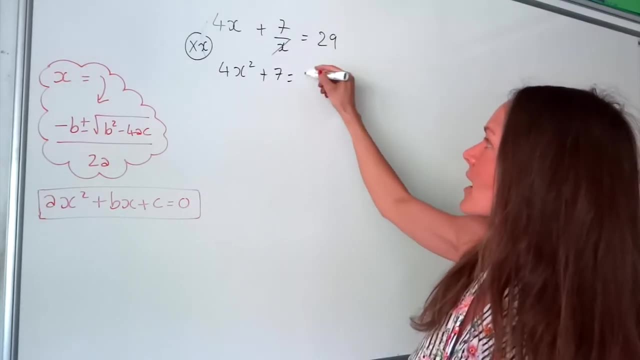 I multiply this by x, I get 4x squared. If I times this by x, well, it just cancels and I'm left with 7.. And if I times this by x, I get 29x. Now, remember, we can only start using this formula. 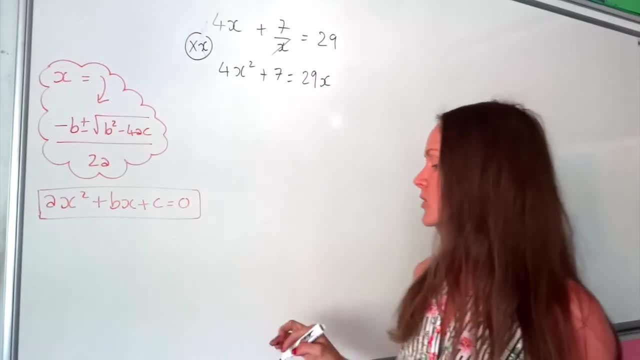 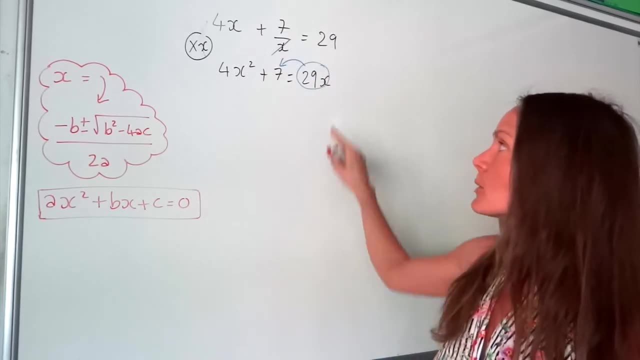 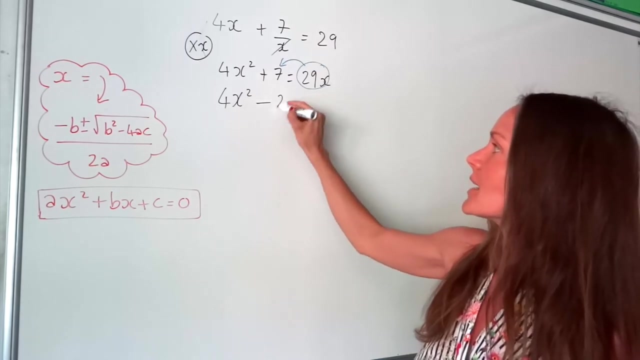 if our quadratic is equal to zero. So the next step is to move that positive 29x over to the left-hand side of the equals so that we've got zero left over. So remember, whenever it moves across the equal sign, it changes signs, it becomes negative. Everything else stays the same. 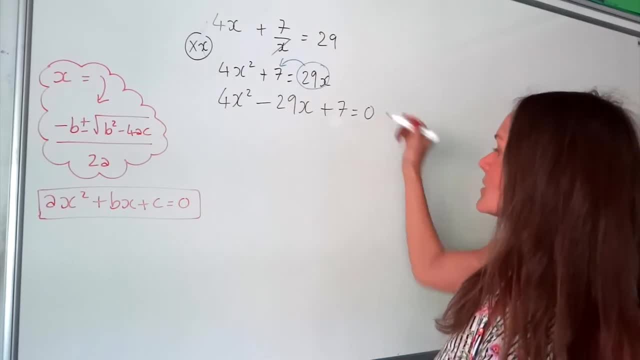 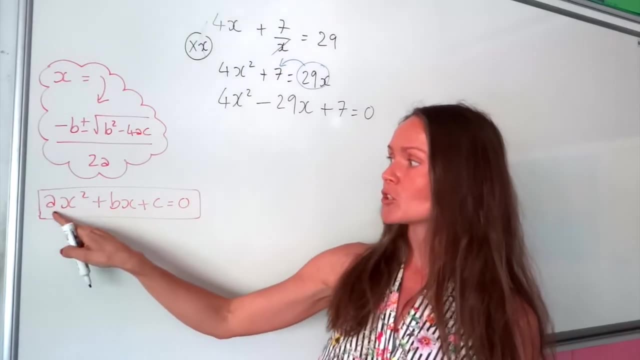 so this is still positive 7.. And now I've got equals zero. So next, just like before, we can identify our values of a, b and c. a is just the coefficient of x squared, So here it would be positive 4.. b is the number in front. 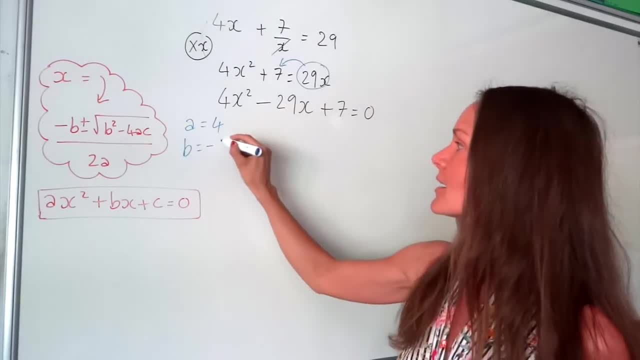 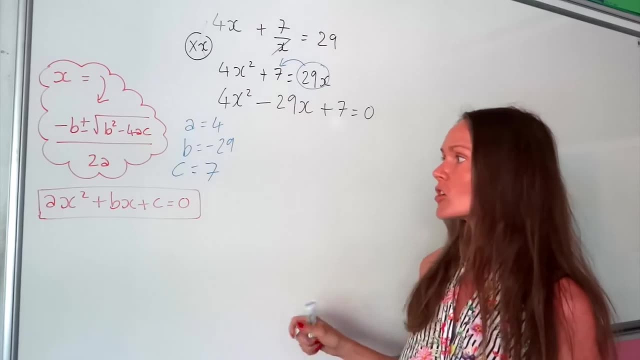 of the x. So here, negative 29. Don't forget that sign. And c is the number by itself, so positive 7.. And just like before, you're just doing substitution, You're just putting these values into the formula. So now I'm going to multiply this by x squared. So if I times this by x, 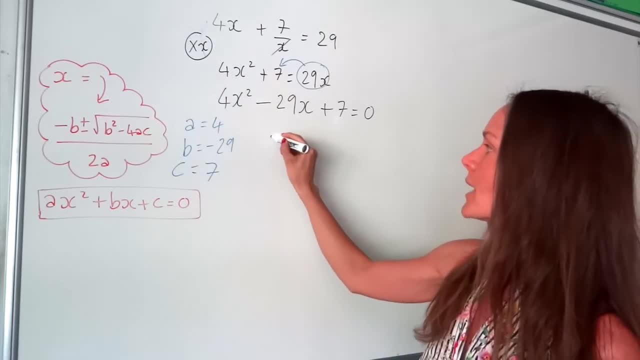 it's going to be negative 2.. So I'm going to multiply this by 2.. So I'm going to multiply this by 2.. So now you have the formula. So minus b. Well, we have to write minus And then be careful.